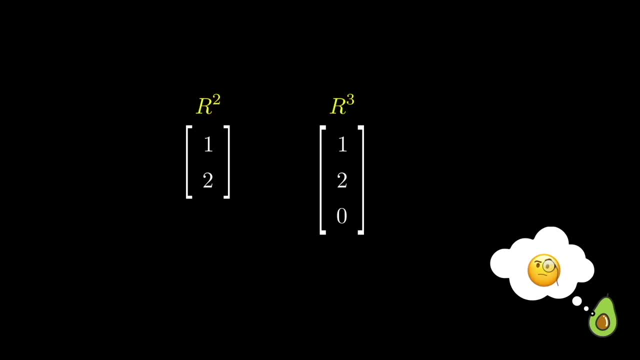 My teachers say the left one is in R2, the right one is in R3.. I used to think those are the same thing. I mean they both have one for x, two for y and they got nothing for z. But that's not the case. They both have one for x, two for y and they got nothing for. 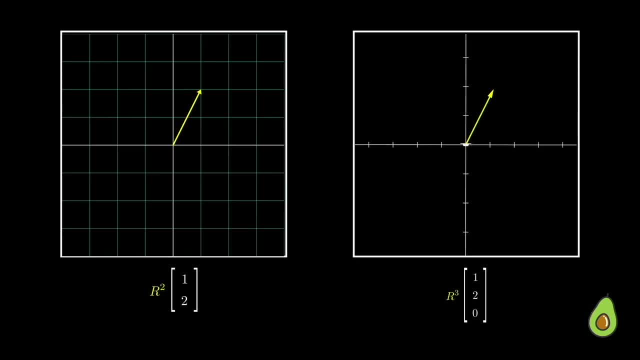 z right. Even if we do represent them on a graph, they look so much similar. I go ahead asking the vector on the right about its z value. It said, oh, zero. I go ask the z value of the left vector. It got very confused, having no idea what a third dimension is ever. 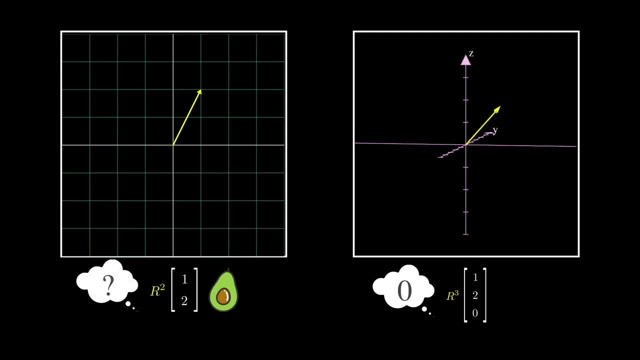 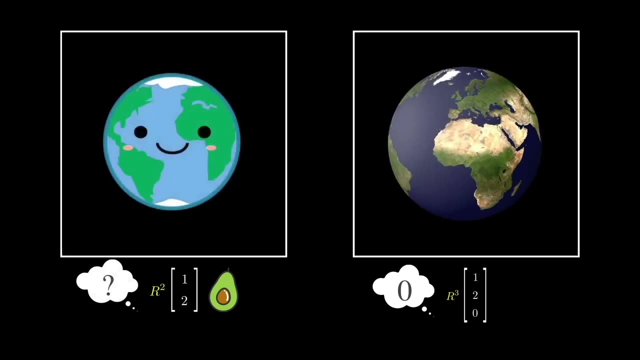 like. In addition, I can go nudge the R3 vector around such that the z value is no longer zero. But for the R2 vector, no matter how I rotate stretch scale, it is always devoid of z. Despite looking similar, in reality there are completely different species that live in. 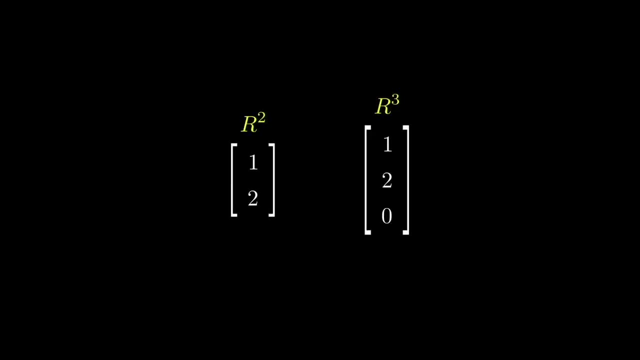 different dimensions of the universe. If those two types of vector are so different, is there a mechanism which can transform one to the other? And that's the power of rectangular matrix. In particular, a 2x3 matrix has the ability to take a vector in R3, transforming that down to 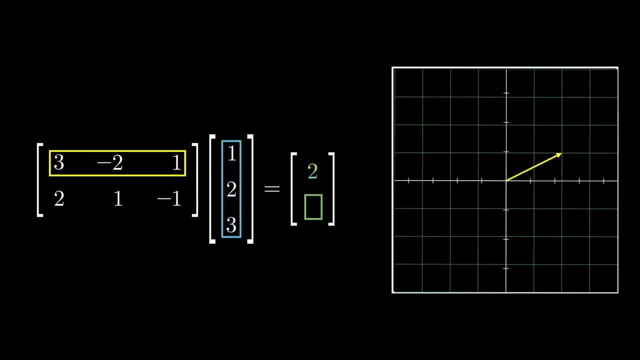 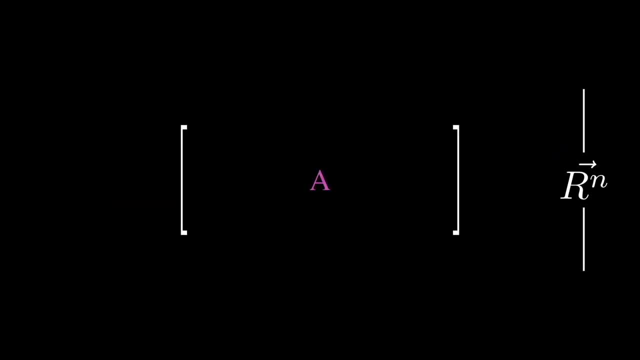 a vector in R2.. Makes quite a lot of sense if we just look at the matrix vector multiplication. A matrix of size n by n has the power to transform a vector in the nth dimension to a vector in the nth dimension. This is why we say matrix apply a linear transformation. 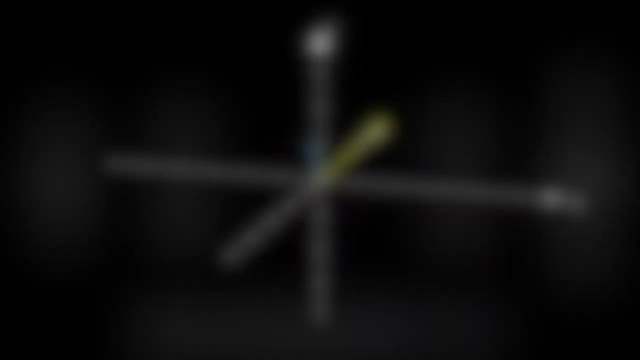 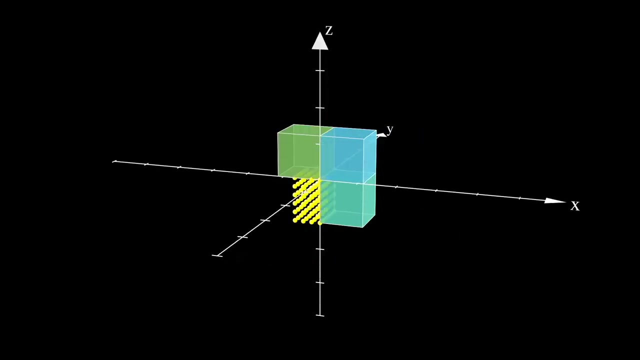 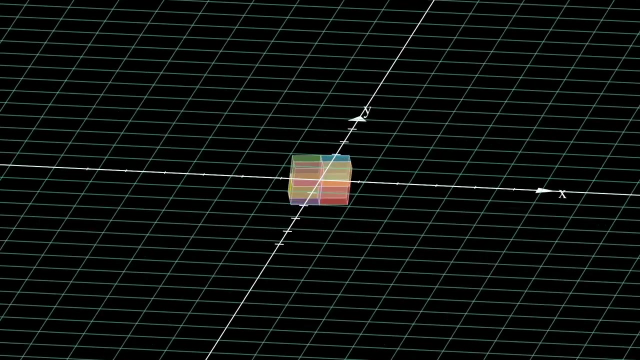 from Rn to Rm. Remember we can represent vector as arrow and represent arrow as dot and a collection of dots as object. Simply illustrating the visual of a matrix is simple, but the process of interpretation is hard. The visualization of rectangular matrix gets very confusing, so it's good if we try to understand. 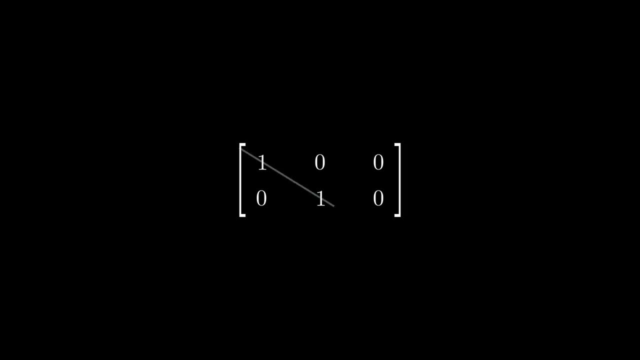 the simplest case first, which is this matrix. You see, it's similar to the identity matrix by the rectangular version of it. For the context of this video, let's give it a cool name: the dimension eraser. This matrix here represents the simplest form of linear transformation. 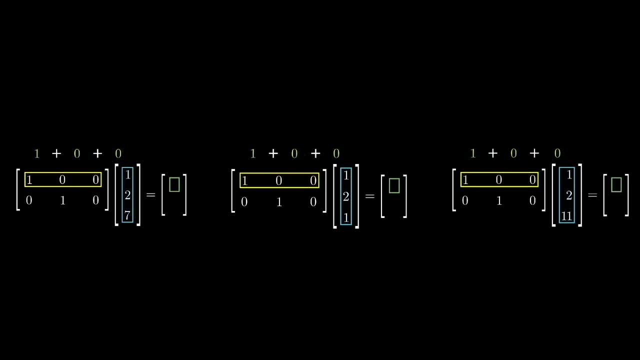 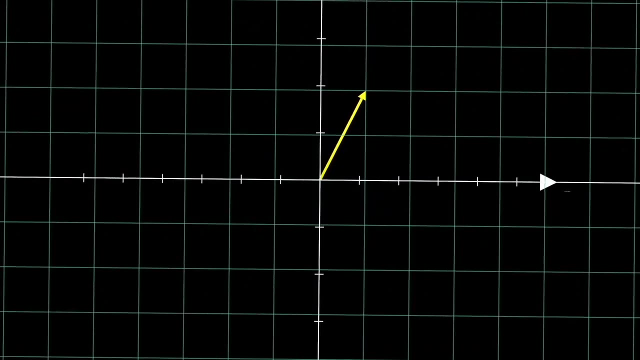 from R3 to R2.. Its multiplication with any vector always preserve the x and y, but completely remove the z value, regardless of the initial z. So what this means is that, for example, the vector in R3, we can map down to the vector. 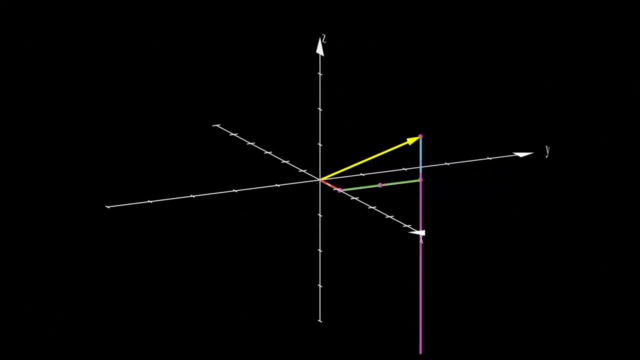 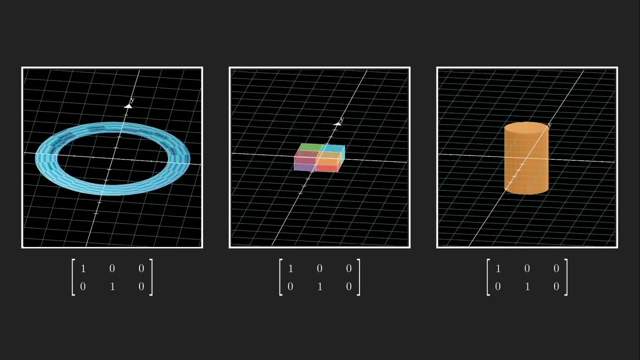 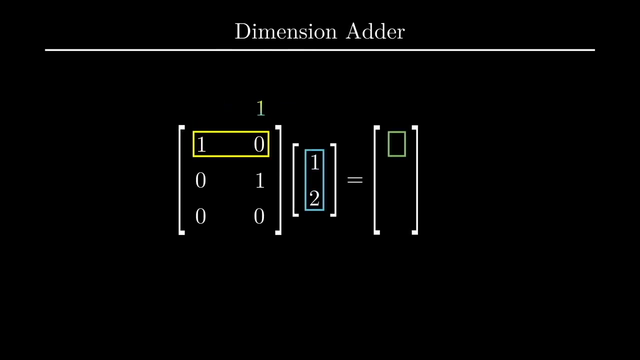 but all the vector in the form of any z transforms to. We can also have something like dimension adder. For example, this 3x2 dimension adder here basically appends 0 as a z value for whichever input R2 vector. 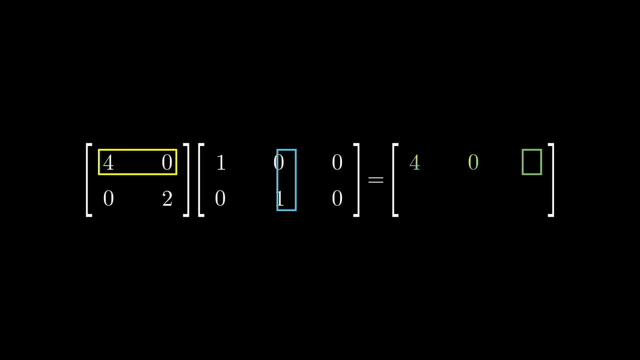 Oh, actually, I think here is a good place for me to show you a composition from R3 to R2.. Whenever we multiply a matrix and a matrix, we essentially combine their distinct linear transformations. Here we can multiply the dimension eraser with its diagonal matrix. 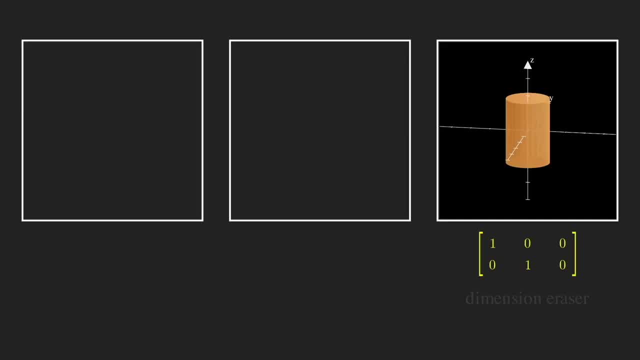 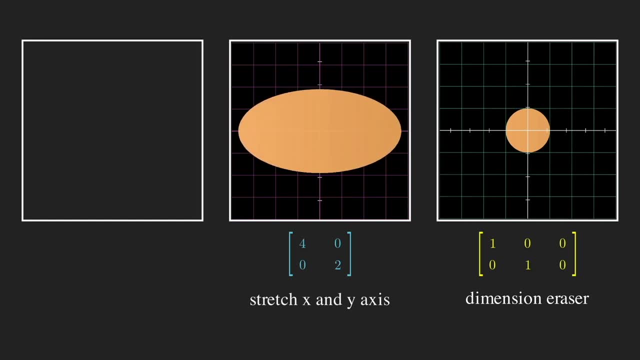 and let's call this product matrix The matrix C. The dimension eraser takes away the third dimension and then, diagonal matrix, stretches the x and y axis accordingly. The matrix C, since it's a composition of the two matrices on the right. 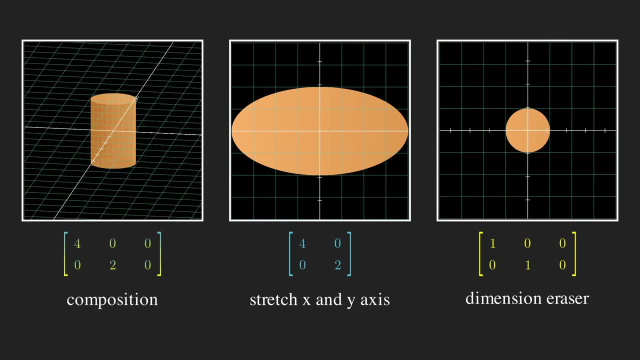 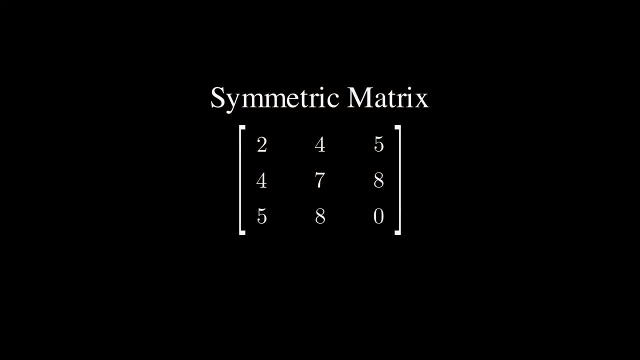 would basically encapsulate the two transformations, but in just one go. Chapter 2 flashback. Symmetric matrix is a square matrix in which on two sides of the diagonal the entries are identical. It has a very strong property which almost no other matrices have. 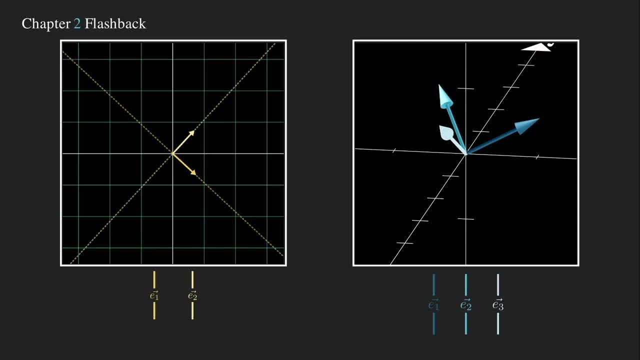 The eigenvectors of symmetric matrix are perpendicular to each other. so that means if we normalize the eigenvectors and package them into a matrix, we get an orthogonal matrix which implies rotation. The transpose rotates the eigenvector to align with the standard basis. If we don't take the 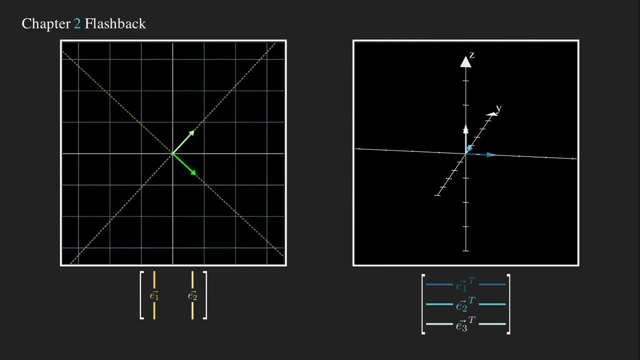 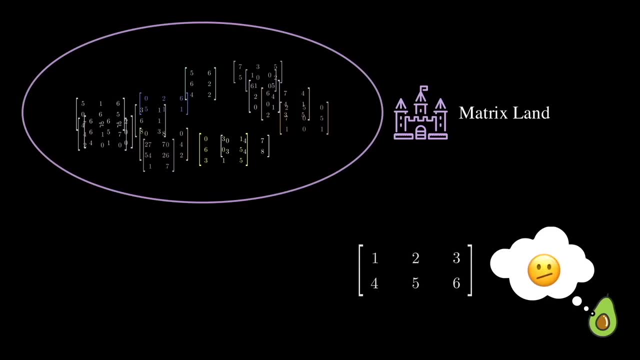 transpose that matrix rotates to the standard basis. so we get an orthogonal matrix which implies rotation To the eigenvector. Symmetric matrix is nice, we gotta take advantage. Yet everyone knows most matrices in nature are not symmetrical. 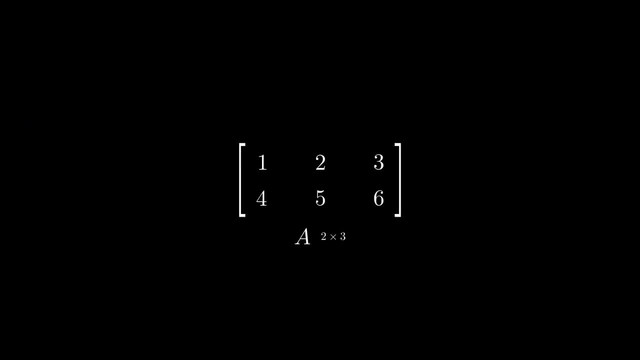 But we just happen to have the ability to artificially construct symmetry out of nowhere. Consider this matrix here, which is obviously not symmetrical. If we take the transpose and multiply them together, we get a square matrix, But also symmetric. We can also put the transpose on the left and do the multiplication. 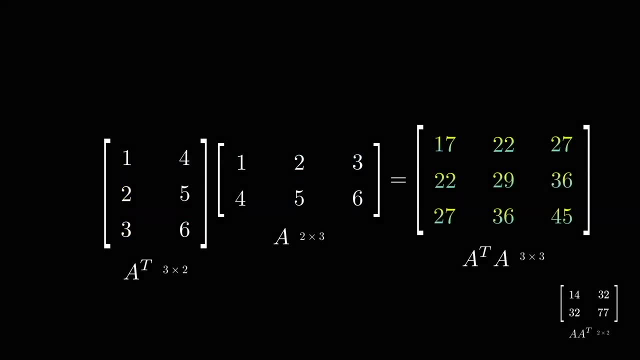 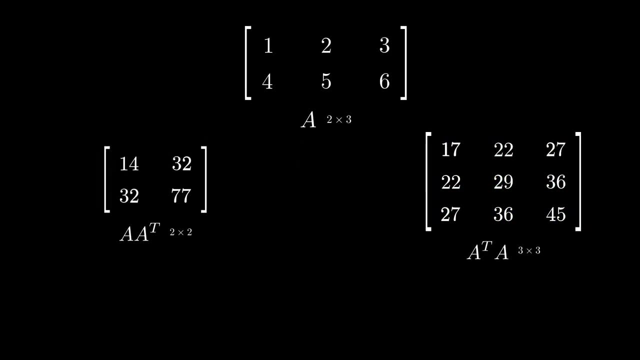 We once again see a square matrix that is also symmetrical. It's good to take a moment here to appreciate we just created two symmetric matrices from a rectangular matrix A. In general, this is true for any matrix A which AA transpose. 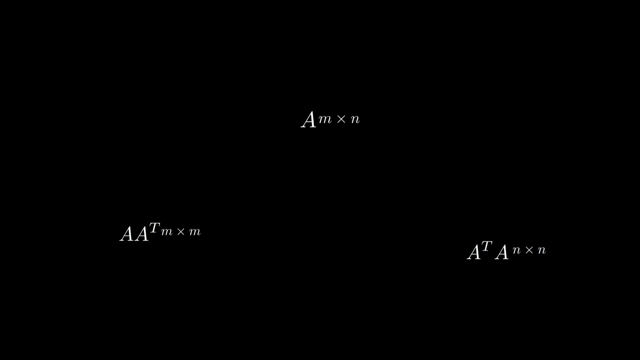 and A transpose A are symmetric matrices. See if you can prove this statement on your own. For now, we stick to the concrete case when A is 2 by 3. And let's give them some meaningful names as well, Since they're symmetric matrices. 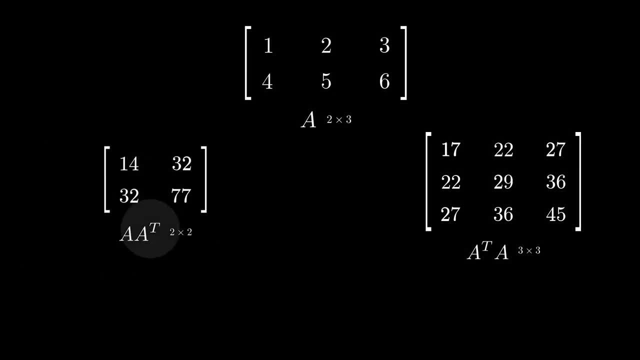 the letter S better be in there. Let's call AA transpose S left and A transpose A S right. I know that you know S left and S right are symmetric matrices, So S left would have two perpendicular eigenvectors in. 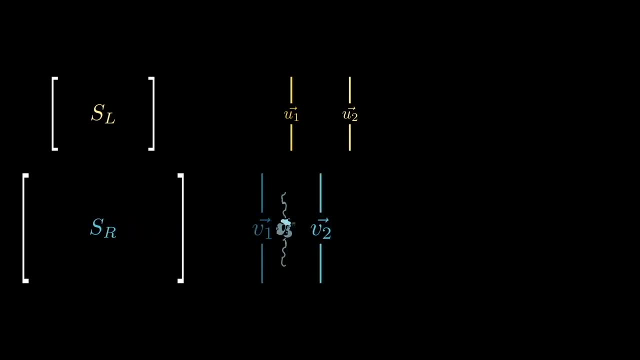 R2, and S right would have three perpendicular eigenvectors in R3.. Since all those eigenvectors are closely related to the original matrix A, we have special names for them as well. The eigenvectors of S left are known as the left singular vector of A, And likewise the eigenvectors of S right are the. 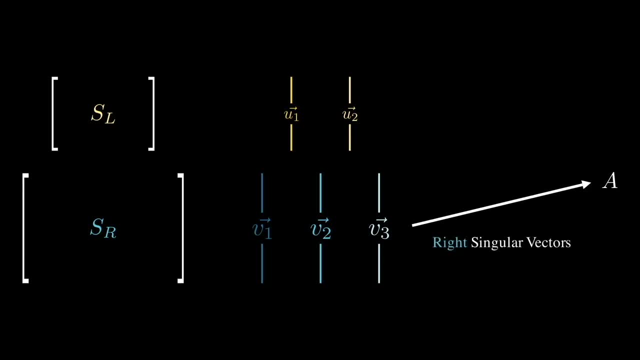 right singular vector of A, And likewise the eigenvectors of S right are the right singular vector of A. The actual right singular vector of A is the right singular vector of A. Up next, I'm about to provide two facts, without going to the detail. 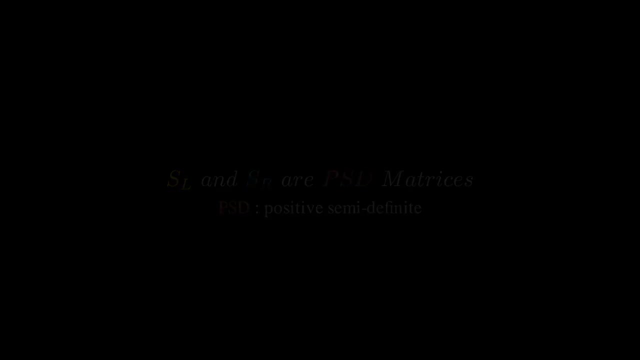 S left and S right are known as PSD matrices. This implies the eigenvalues for each eigenvector are non-negative. The second fact which is not obvious: if we sort the eigenvalues in descending order, for both set, the overlap ones are numerically identical. The biggest eigenvalue 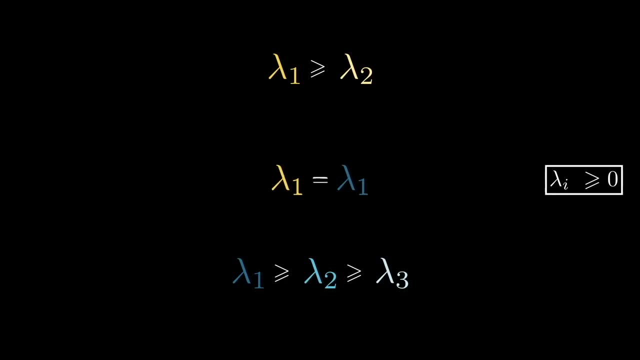 of S left equals to the eigenvalue of S right, which is known as PSD, And so the eigenvalues of S left are non-negative to the biggest eigenvalue of S-ray and so forth. The leftover eigenvalue is guaranteed to be zero. 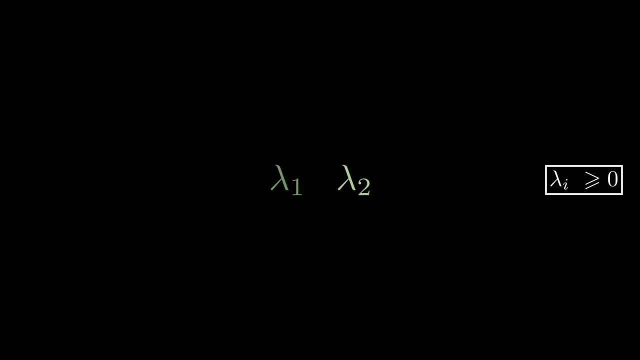 Just like the singular vectors, those shared eigenvalues are indirectly derived from the very original matrix A. If we take their square root- and, my friend, those are the singular values of matrix A- A lot of things we did so far seem random. We have ambiently collected all pieces. 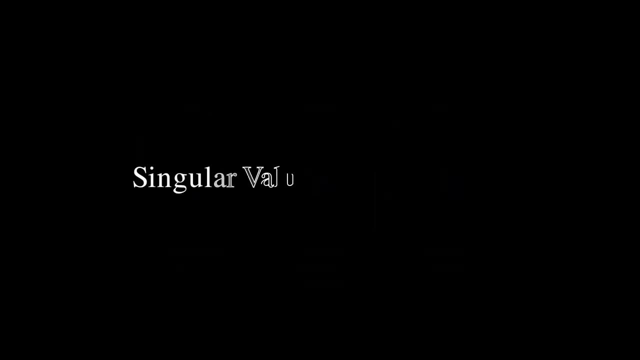 of knowledge which we need to understand. SBD Now behold its entrance Once again. any matrix A can be unconditionally decomposed into three very special matrices in which the matrix sigma is rectangularly diagonal. the matrix V and U are orthogonal. 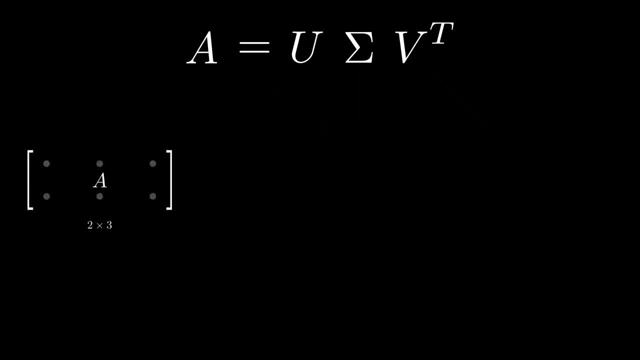 also known as orthogonal matrices. But what exactly are they exactly? The matrix sigma would have the same dimension as matrix A. The numbers on the diagonal are the singular values of matrix A, arranged in descending order. every other entry is zero. The matrix U contains the normalized eigenvectors of S-left, which are rearranged. 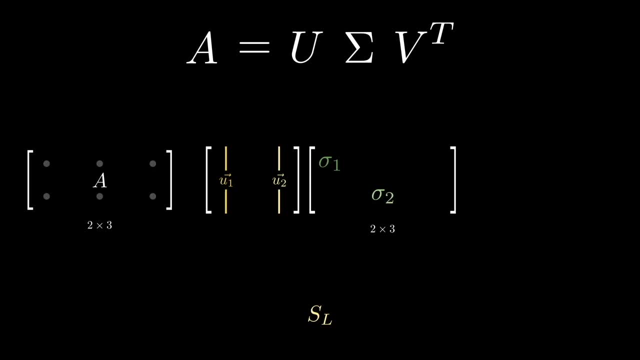 in descending order of their eigenvalues. Another way of saying this is the left singular vectors of matrix A. On the other hand, matrix V contains the normalized right singular vectors of matrix A, also arranged in descending order, and then we transpose that to get V transpose And remember this. 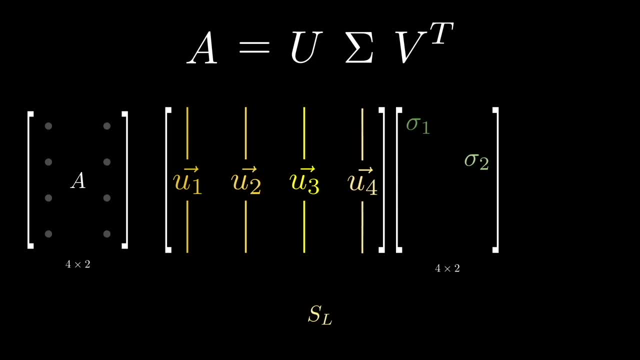 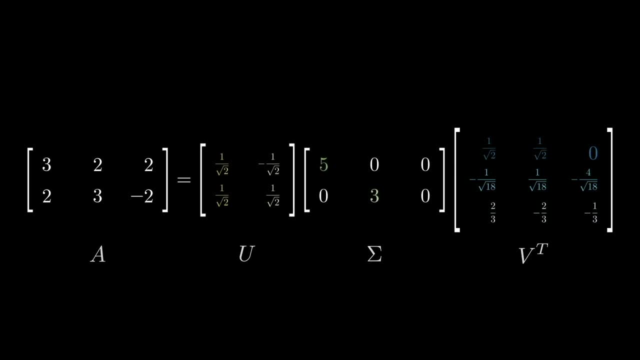 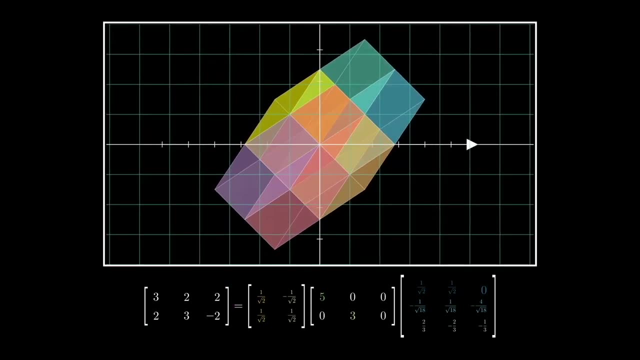 generalizes to all kinds of matrix A. The moment I've been waiting for the visualization. The matrix A here by itself applies a complicated linear transformation from R3 to R2. But we know using SVD it can be perfectly understood as sequentially applying the. 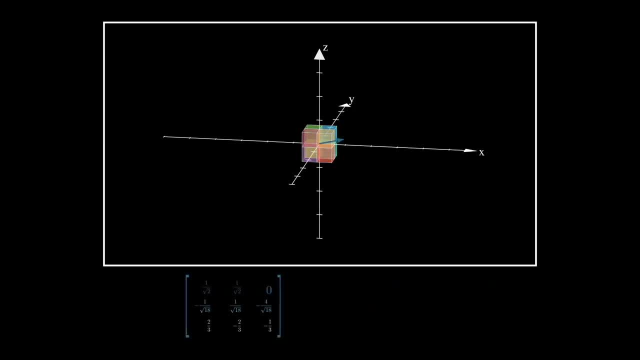 three simple matrices on the right, The blue matrix, or V transpose, is an orthogonal matrix which applies a rotation such that the right singular vectors return to the standard basis. So, more precisely, the singular vector with the biggest singular value lands on x-axis. the singular vector with the 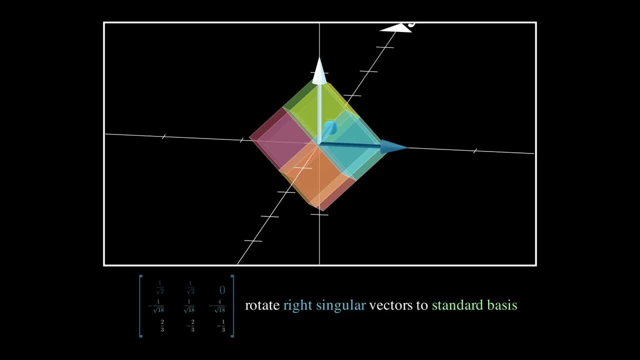 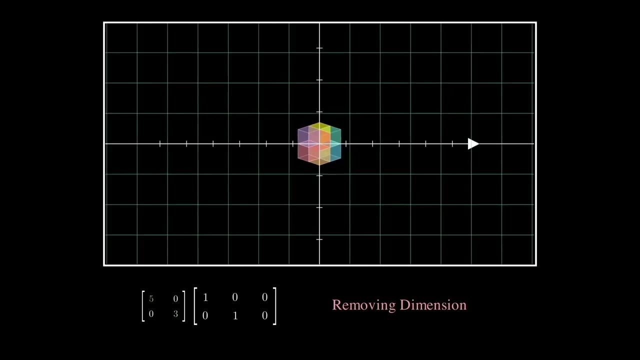 second biggest singular value goes on the y-axis and so forth. The matrix sigma is rectangularly diagonal and it's essentially a square diagonal matrix composed with a dimension eraser. The dimension eraser is removing the third dimension and see that the diagonal matrix stretches x and the y-axis based. 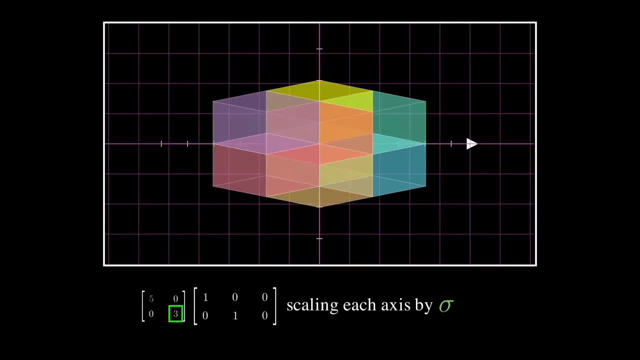 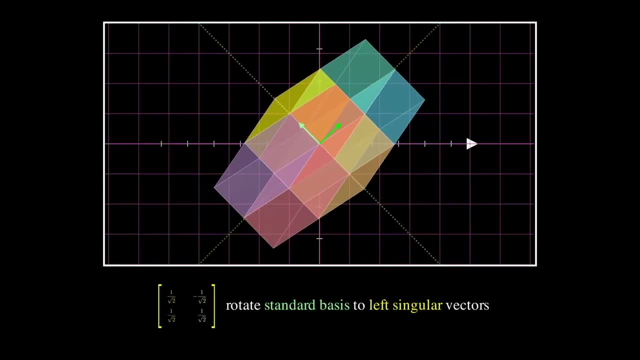 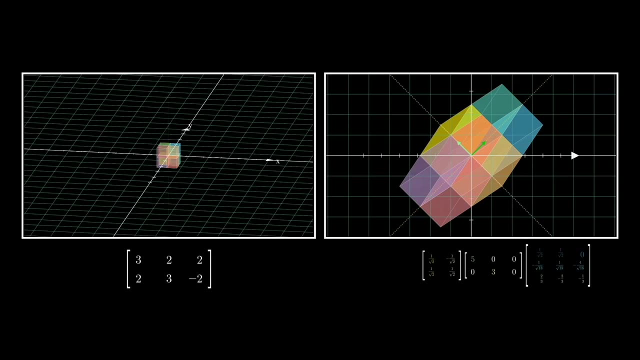 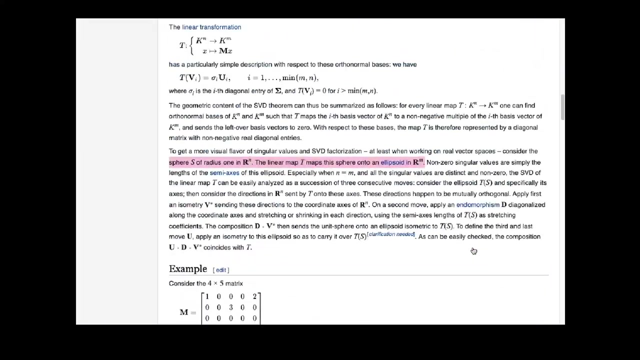 on the singular value. And the final step: the matrix U rotates to standard basis to align with the left singular vectors. And boy you bet those transformations composed is exactly the same as A. So Wikipedia said a few things about the visual flavor of SVD, that any matrix 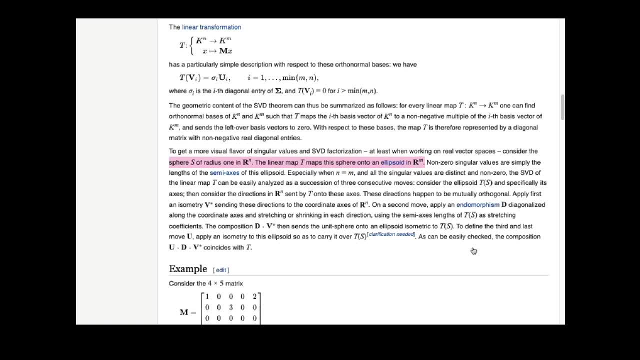 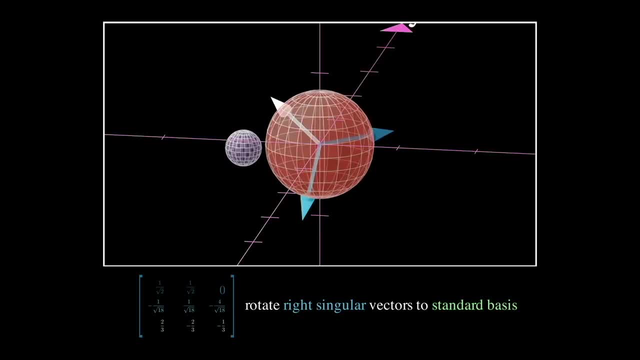 essentially just maps sphere into ellipsoid across different dimensions. Let's see for ourself. After singular value decomposition, the first step of any linear transformation is also a linear transformation. There's always a rotation in Rn. If you rotate a sphere, it's still a sphere. 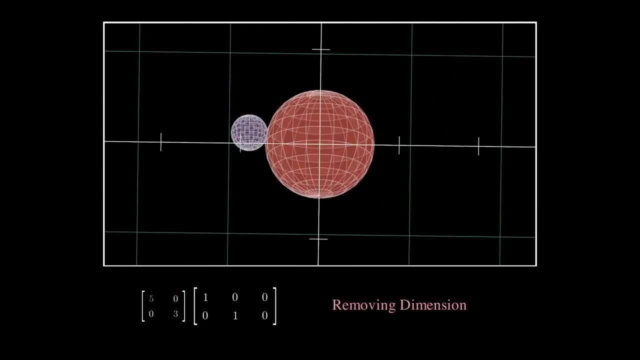 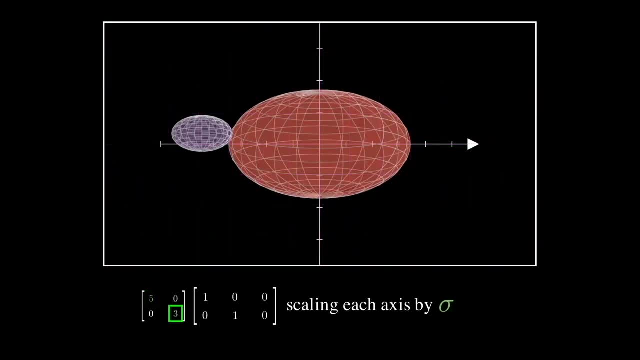 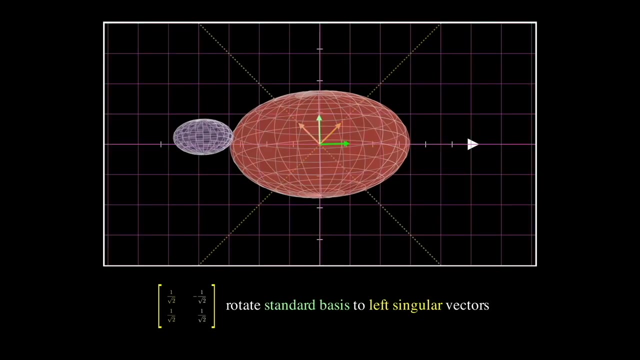 Taking away the third dimension of a sphere in R3, makes it a circle in R2.. Stretching uniformly along the x and y-axis makes a circle an ellipse And the final rotation still preserved the geometry of the ellipse, just changing that. 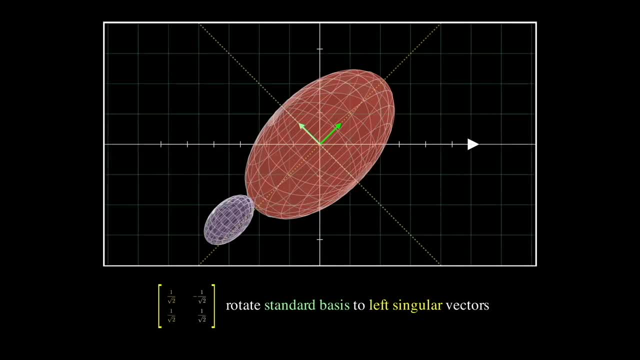 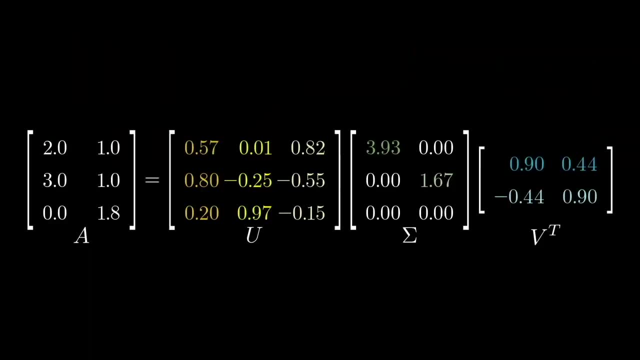 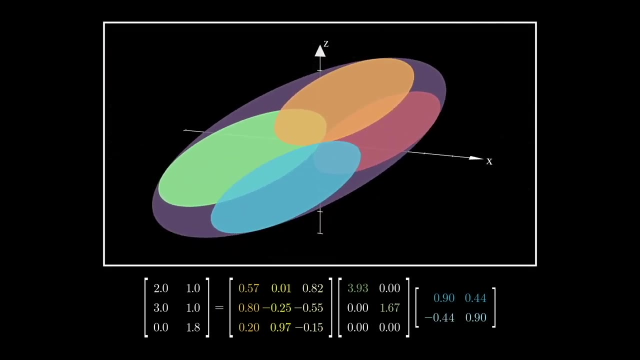 to a different position in R2. And by no means that was an rigorous proof, but certainly some intuitions. And lastly, let's look at an example of a linear transformation from R2 to R3. The spirit of SVD very much still holds. Firstly, we begin with the rotation in R2.. 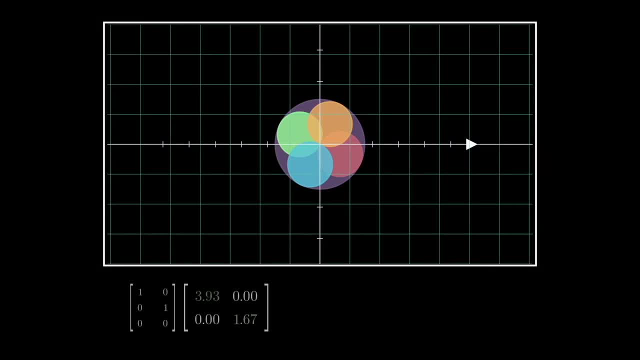 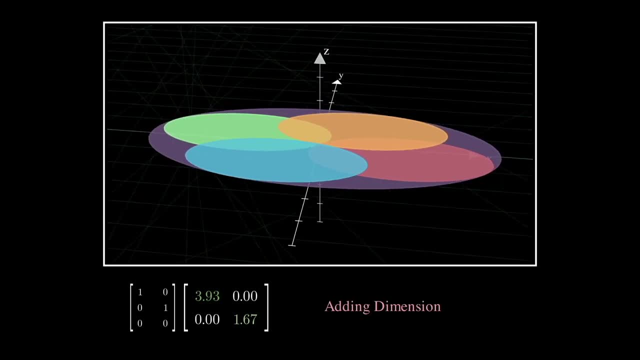 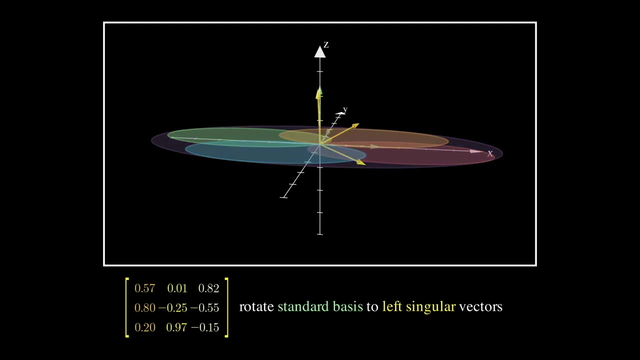 But next, since the matrix sigma is 3 by 2, we scale based on the singular values, And then we're adding a new dimension And finally we rotate the standard basis- x, y, z- to align with the left singular vectors. 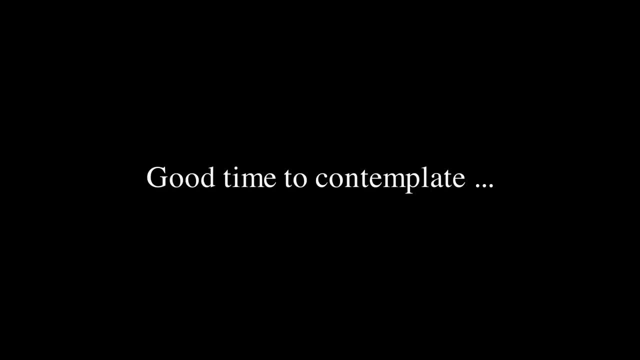 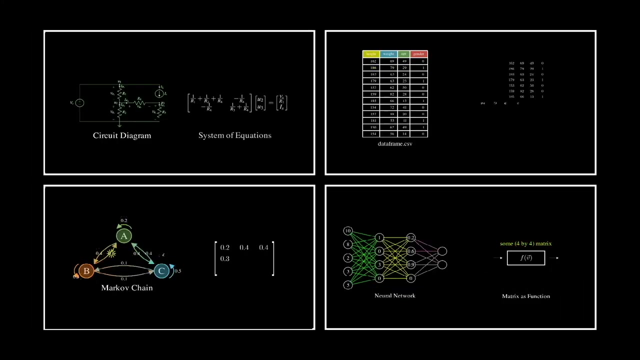 This video should end now. Nonetheless, it's good to contemplate on a question: Is the entire purpose of SVD to decompose linear transformation into those four sequential actions? Is our visualization, the correct interpretation of SVD itself? Not exactly. I mean. what even is a matrix? to begin with, This mathematical object has 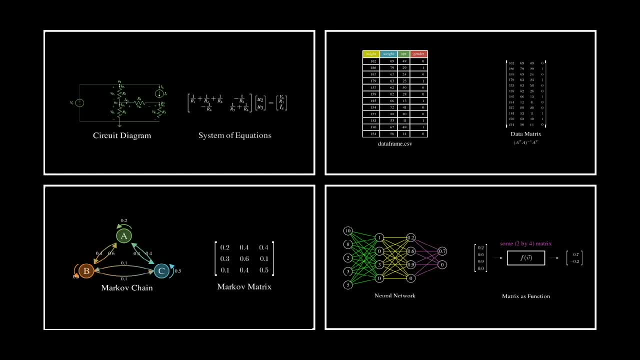 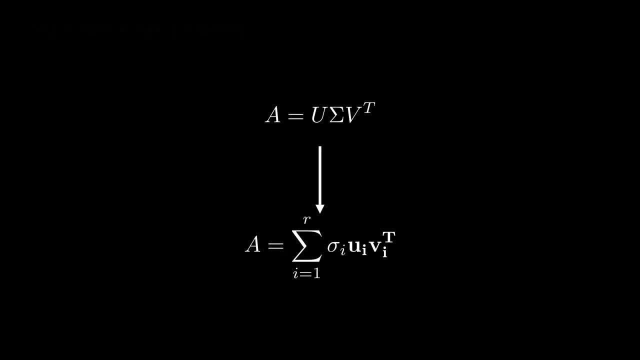 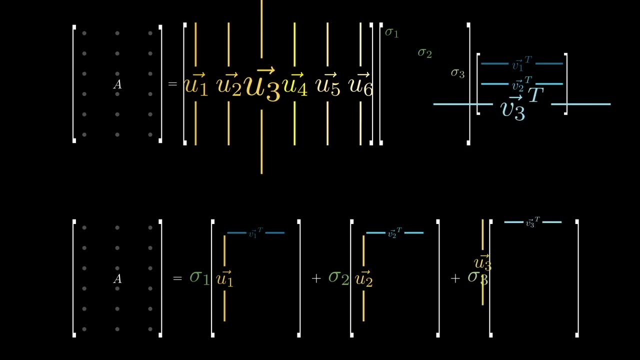 different interpretations under different contexts. The same matrix can mean very different things to different people. Another popular interpretation of SVD is to view a high-rank matrix as a summation of rank-one matrices. An application of this is low-rank approximation. We can view a picture. 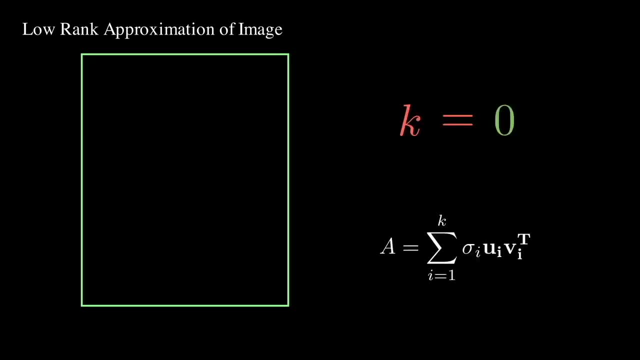 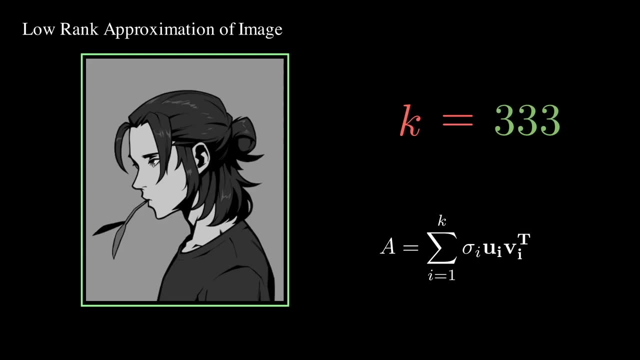 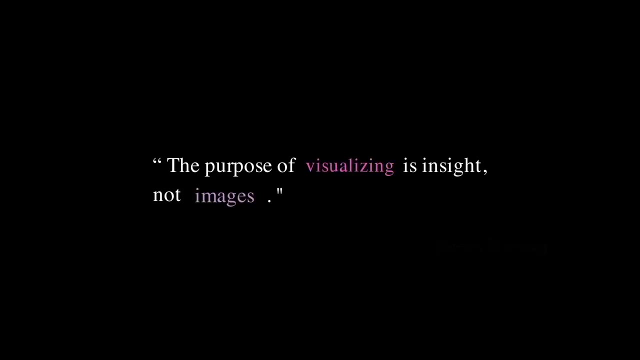 as a massive matrix of pixels and gradually approximate that picture by adding more and more rank-one matrices. A wise man once said the purpose of computing is insight, not numbers. I think the same goes for visualizations as well. SVD as a math exercise is an intense 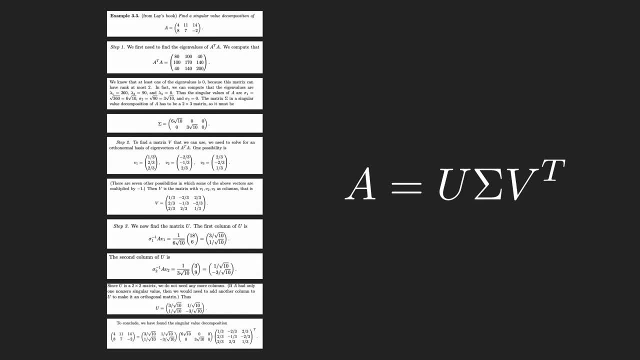 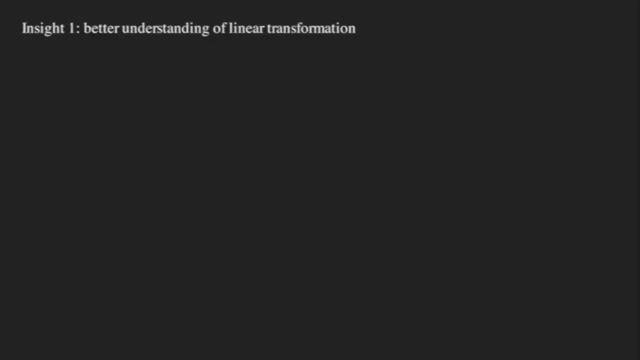 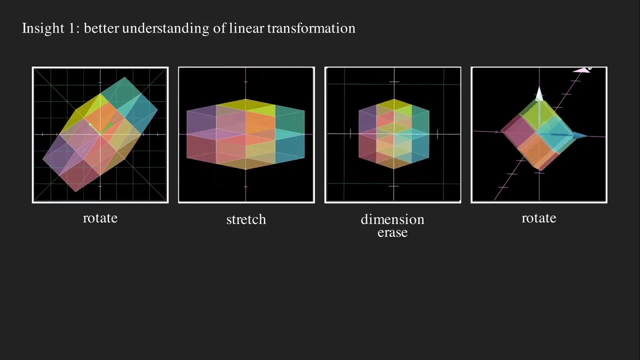 algebraic procedure to follow. Sometimes, after three pages of matrix multiplication and characteristic polynomial, I understood of nothing of what I just did. But decompose and visualize a matrix A into four distinct pieces of simple transformation gives you so much more insights than you'd otherwise have Each, every single step interpretable. 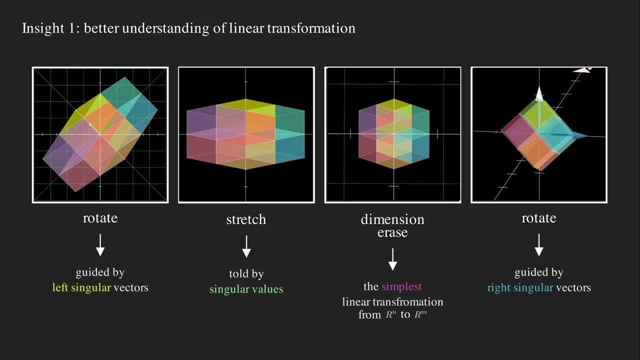 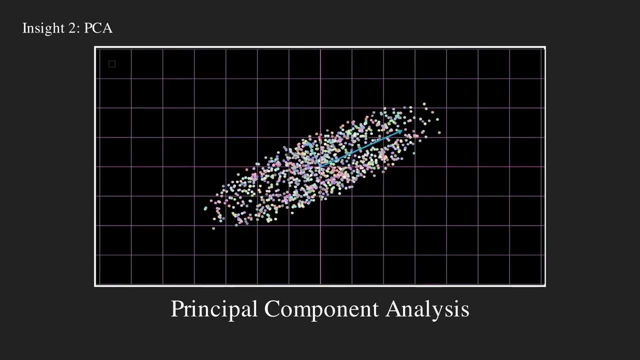 and makes perfect sense. We know precisely what's going on. In particular, that very initial step of rotation from the right singular vector onto the standard basis actually captures the essence of SVD. It's a very simple process, but it's a 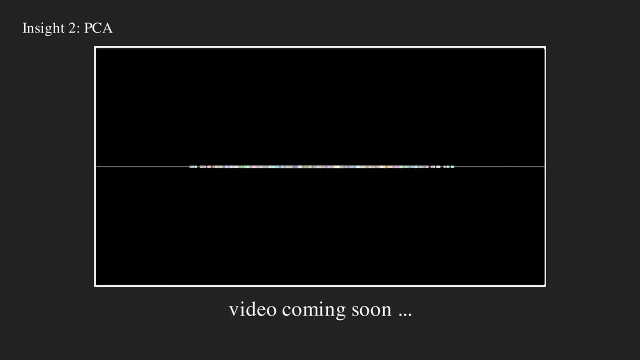 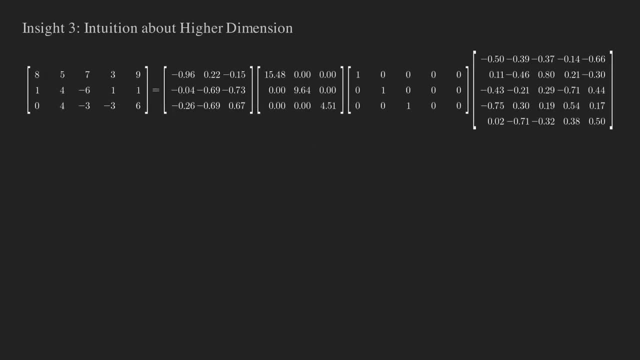 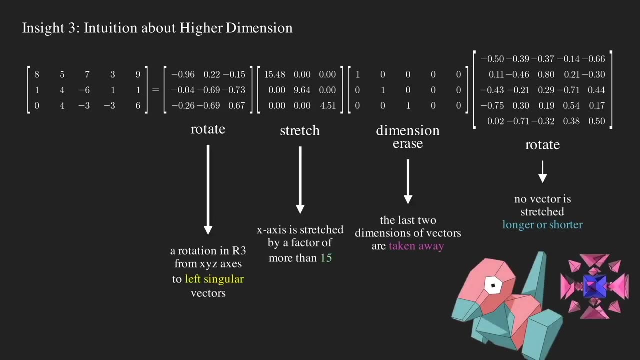 lot of work. I promise a video in the future. Even when things extend beyond the three-dimension, this type of decomposition still gives us a reasonable intuition of linear transformation on vectors, allowing us to say about things which we couldn't see. We know that a rotation does not make things bigger or smaller. Therefore, 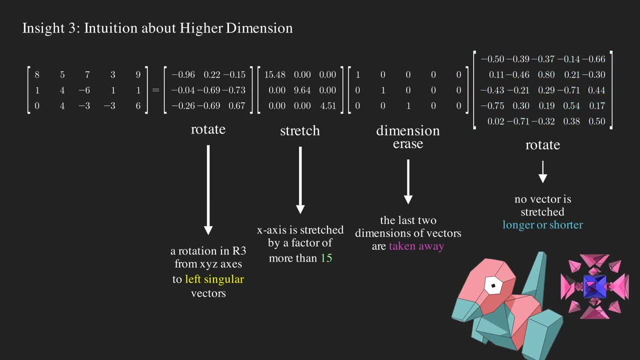 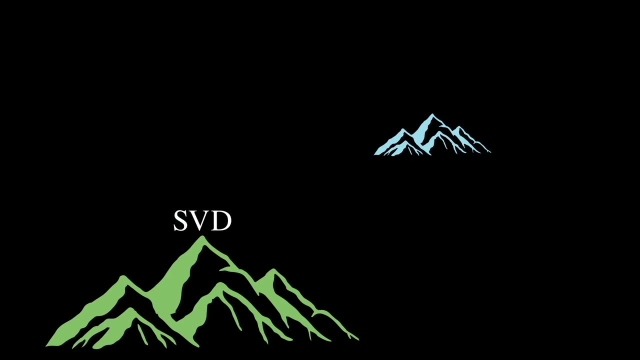 when this matrix acts on higher-dimensional objects, nothing scales, squash blown out of proportion, but pristine rotation around the origin, And after that the last two dimensions of the object is taken away. Sometimes learning the final theorems of a subject is like climbing a mountain. We get. 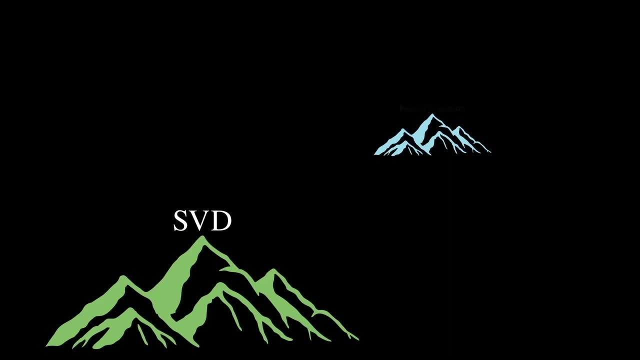 a nice scenery on the top, a higher-level overview, But it's nice to look afar at the other summits and what we see is a Fourier transform. I just want to say some similarity they share about the two monumental theorems: obsession. 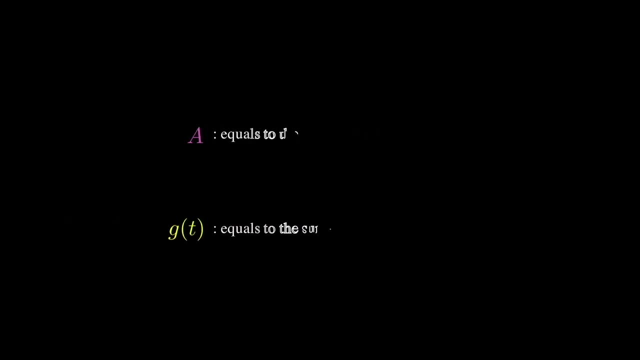 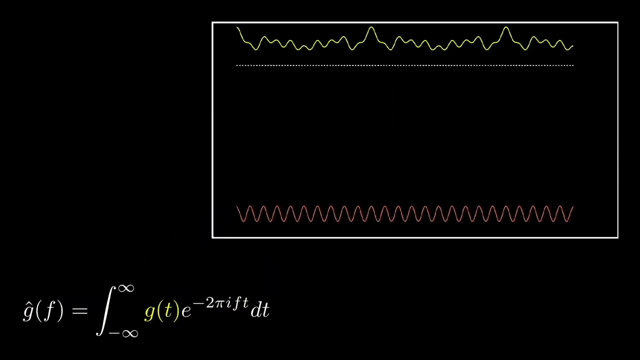 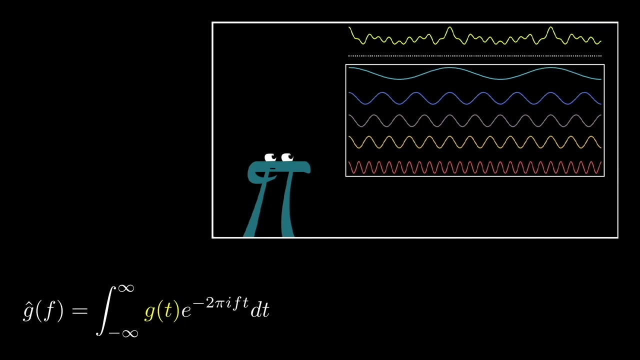 with extreme generalization and linear transformation And decomposition. The Fourier transform is saying any function can be decomposed as the sum of sinusoidal wave functions And when you see the pie creature you already know it's a good video. I left a link here.